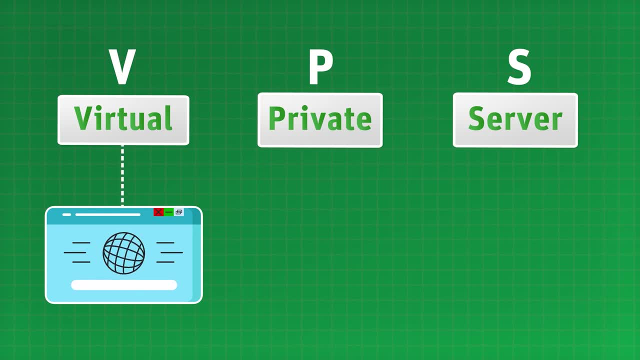 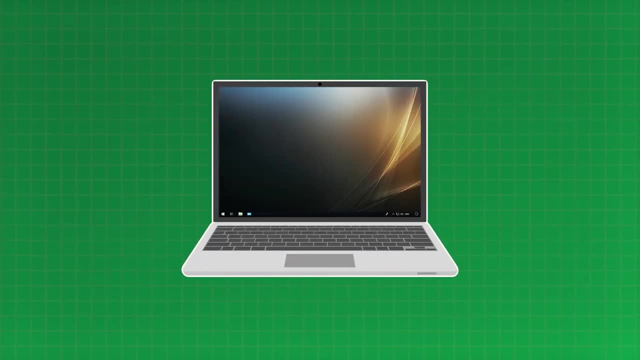 Virtual Private Servers run in a virtual environment that's dedicated just for you and is created on a physical server. For example, imagine you have a physical computer that's being used by four people. It gets annoying really fast With multiple users. all of their files would. 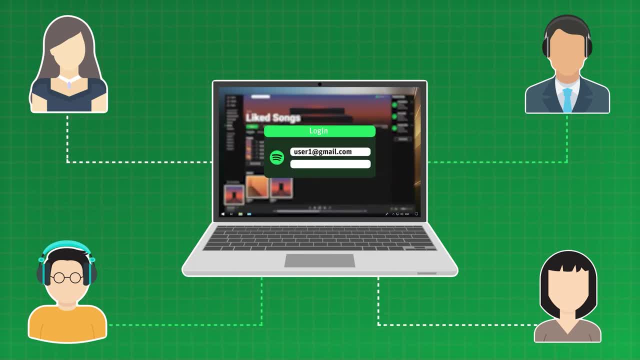 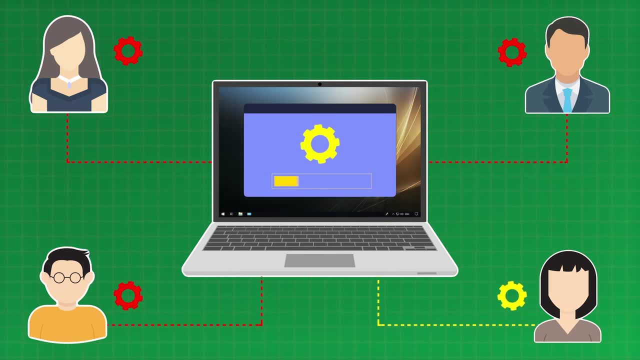 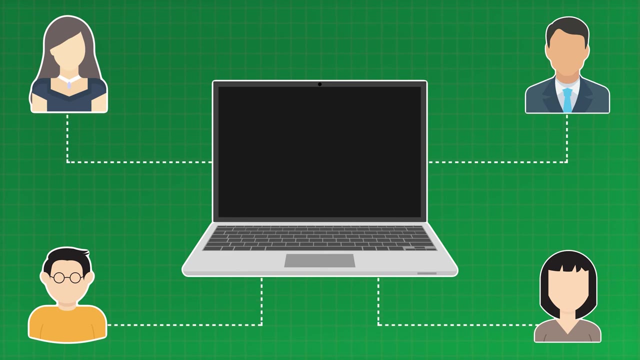 get mixed up. People that want to listen to Spotify have to log out of their previous user's account and then log back into theirs. If one user installs something, everyone has to deal with it and everyone's forced to use the same operating system To solve this. each user can create their own user. 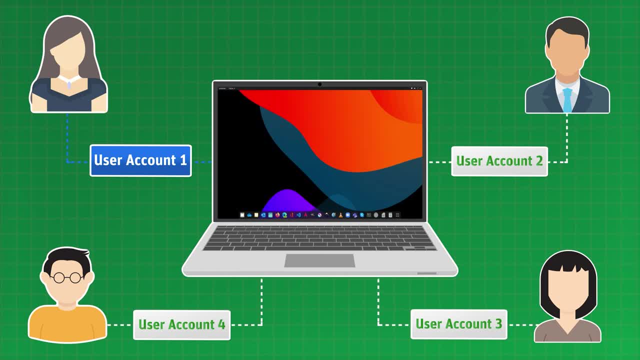 account on the computer with different operating systems and different programs installed. Now, no five-year-old can do that, But if you want to learn more about virtual private servers, files will get mixed up. everyone has a separate account and can enjoy a private experience. 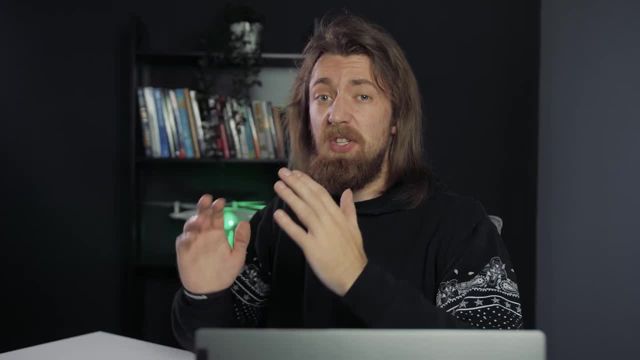 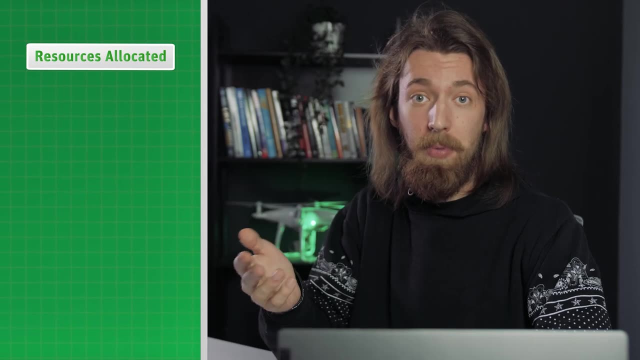 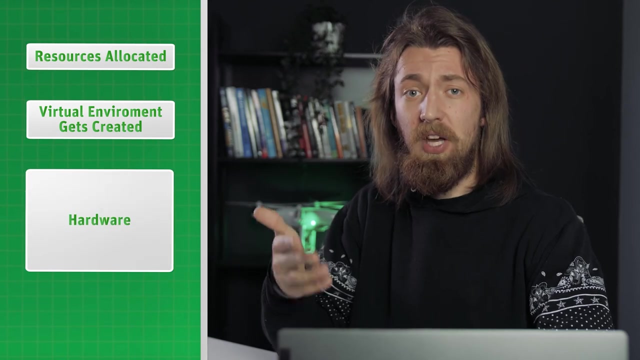 even though they're still using the same computer. This is pretty much how a VPS works. When buying, you tell the provider how many resources you want to use for your website or app. A virtual environment gets created to your specifications. While you still technically use the same hardware, all users have their private little piece. 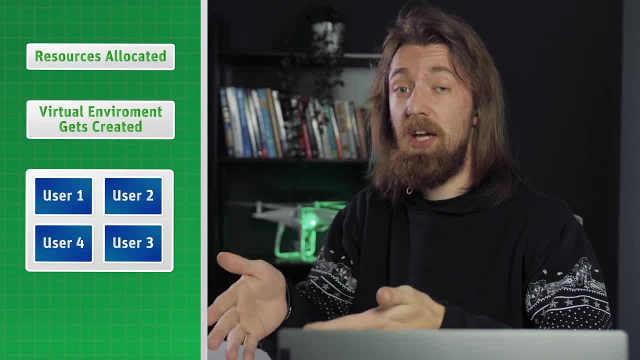 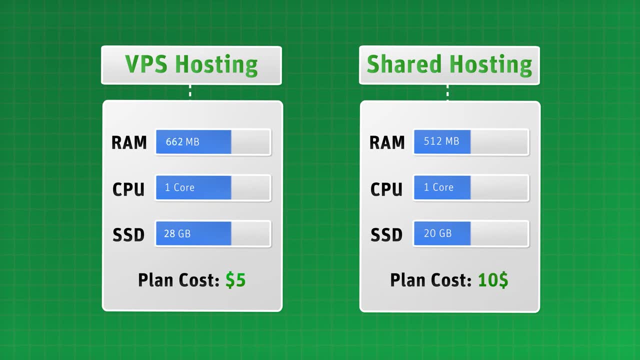 of it and you don't have to fight for space or power with the other sites on that server. And that's not all. Even the cheapest VPS hosting services are usually at least around as powerful or even two times as powerful as the most expensive shared hosting plans. 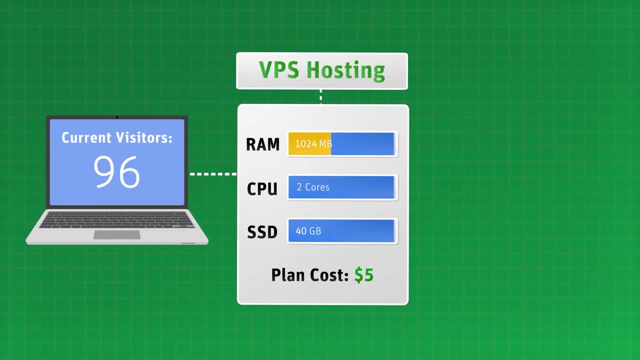 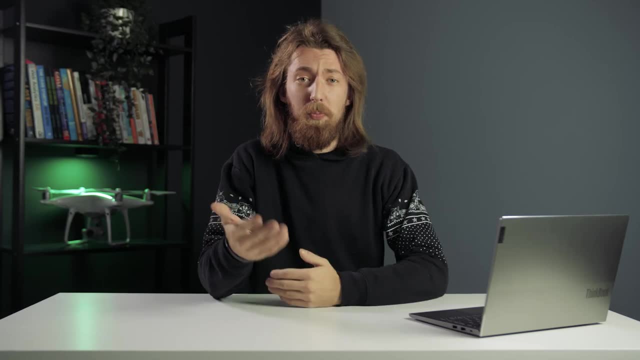 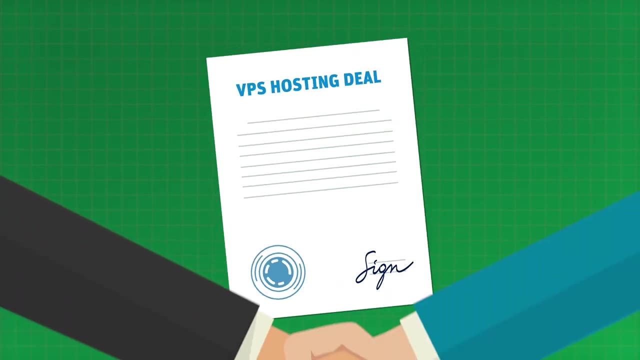 allowing you to have more visitors on your website at the same time and improve browsing speed by loading pages faster. Okay, so why do more people use virtual private servers? Because you can get a VPS service for as cheap as $3 or $4 a month? Well, because in most cases it's not a set-and-forget. type of deal. There are almost unlimited options for customization and most people don't really know what's good for their projects, so they tend to choose suboptimal and expensive configurations. As a non-tech-savvy user, the risk of getting it wrong is just too big compared to the rewards. 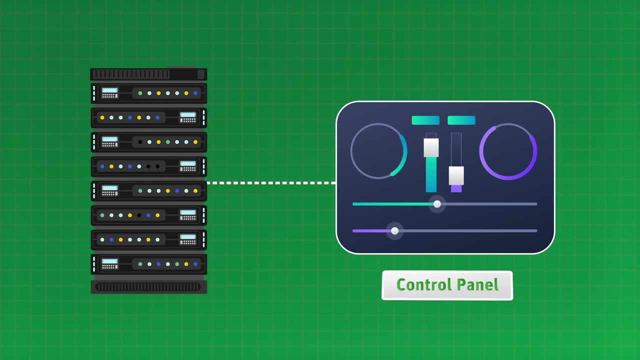 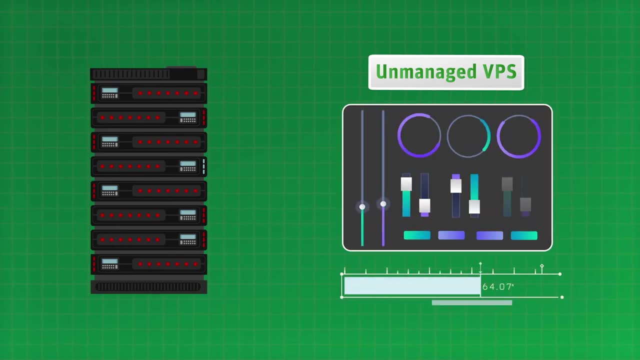 that you're getting. A good example of this complexity would be the control panel. If you're using an unmanaged VPS, well, you don't get one. You either need to install a third-party control panel yourself or manage your server. 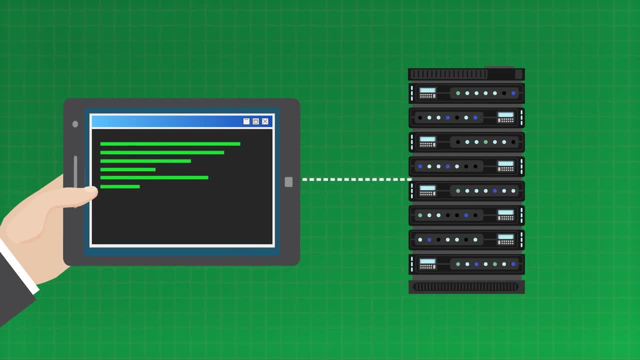 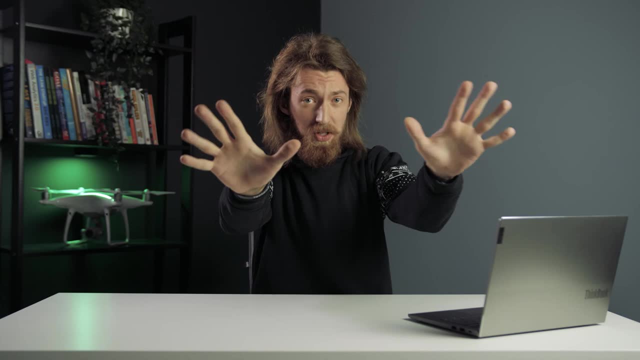 You can manage your server through commands, which is quite difficult, to say the least, And if you misconfigure your server, that could lead to outages and security issues, But that doesn't need to be the case. Notice how I said unmanaged VPS. Well, there's another type of VPS service and it's called